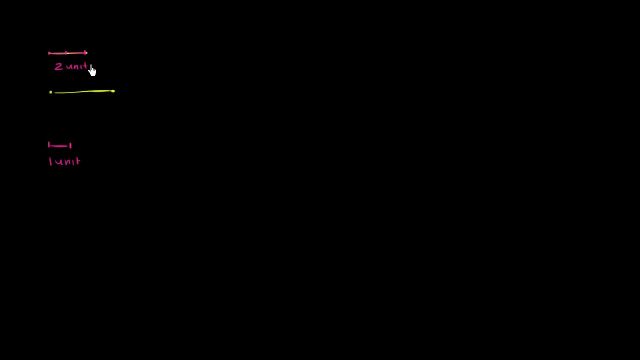 and then we can do it again. So it looks like this is two units, while this third one looks like we can get. let's see, that's one, two, three of the units. So this is three of the units, And right here I'm just saying units. 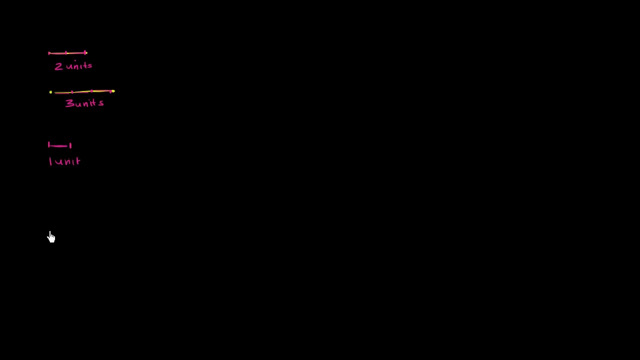 Sometimes we've made conventions to define a centimeter where the unit might look something like this, And it's going to look different depending on your script: We might have a screen, or we might have an inch that looks something like this, Or we might have a foot that I won't be able to fit on this screen. 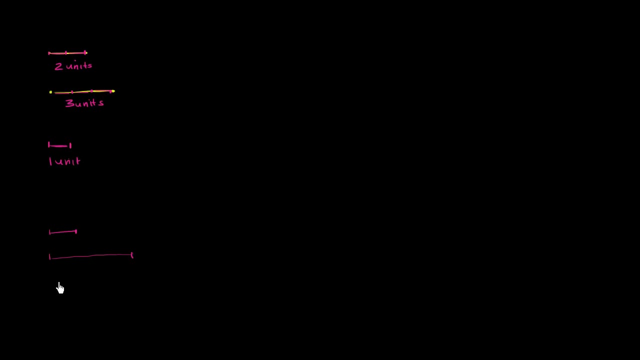 based on how big. I've just drawn the inch or a meter, So there's different units that you could use to measure in terms of. But now let's think about more dimensions. This is literally a one-dimensional case. This is 1D. 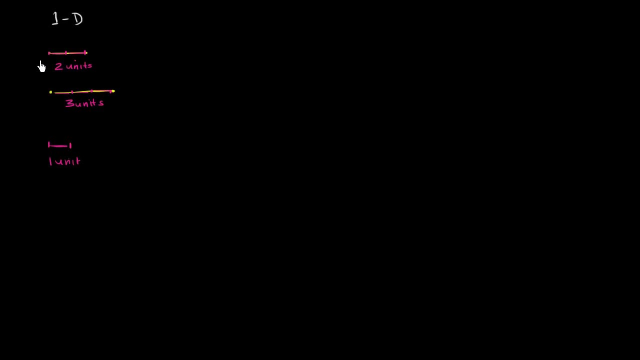 Why is it one dimension? Well, I can only measure length. But now let's go to a 2D case. Let's go to two dimensions, where objects could have a length and a width or a width and a height. So let's imagine two figures here that look like this. 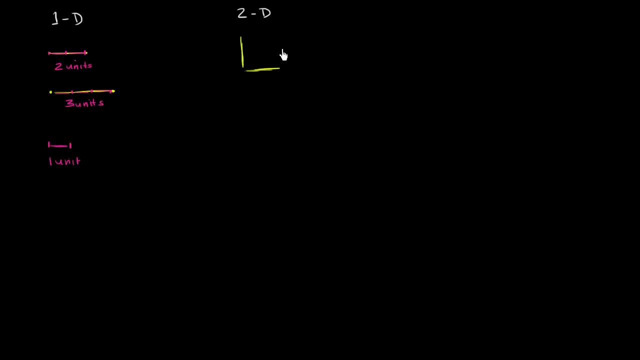 So let's say this is one of them, This is one of them, And notice, it has a width and it has a height, Or you could view it as a width and a length, depending on how you want to view it. So let's say: this is one figure right over here. 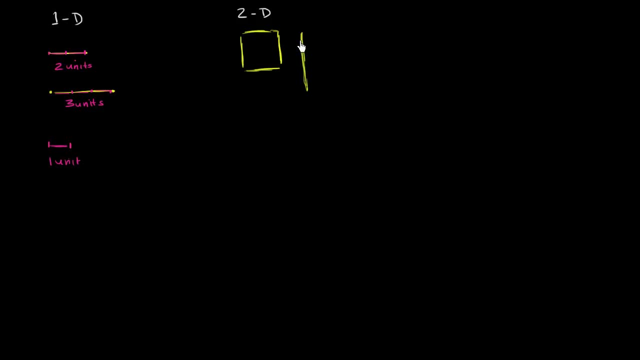 And let's say: this is the other one, So this is the other one, This is the other one right over here. Try to draw them reasonably well Now, once again. now we're in two dimensions And we want to say, well, how much in two dimensions: space. 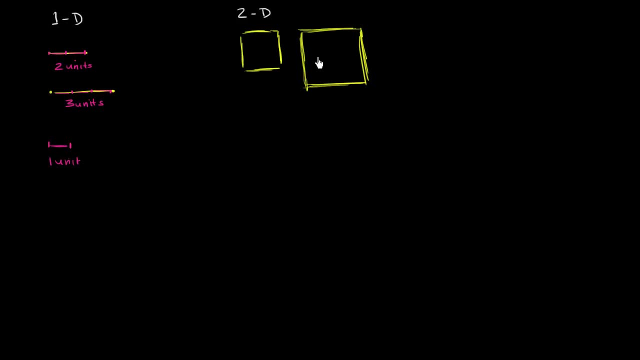 is this taking up, Or how much area are each of these two taking up? Well, once again, we could just make a comparison. This second, if you view them as carpets or rectangles, the second rectangle is taking up more of my screen. 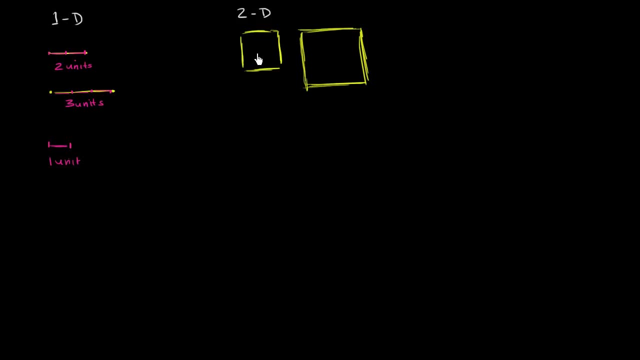 than this first one, But I want to be able to measure it. So how would we measure it? Well, once again, we would define a unit square Instead of just a unit length. we now have two dimensions. We have to define a unit square. 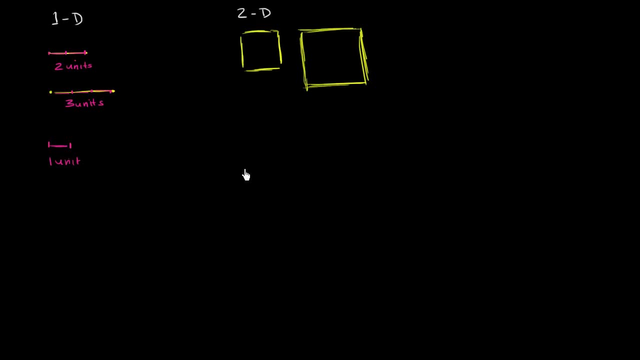 And so we might make our unit square, And the unit square we will define as being a square where its width and its height are both equal to the unit length, So its width is one unit and its height is one unit, And so we will often call this one square unit. 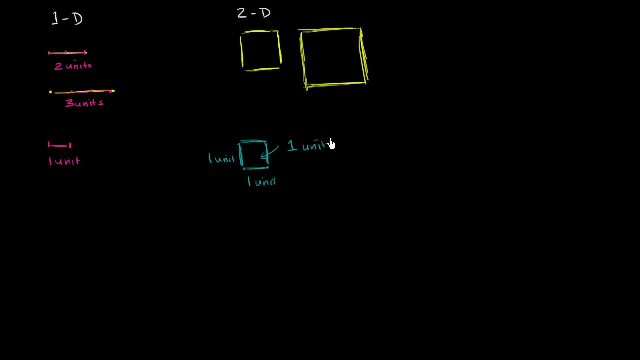 Oftentimes you'll say this is one unit And you put this 2 up here. This literally means one unit squared, And instead of writing unit, this could have been a centimeter, So this would be one square centimeter. 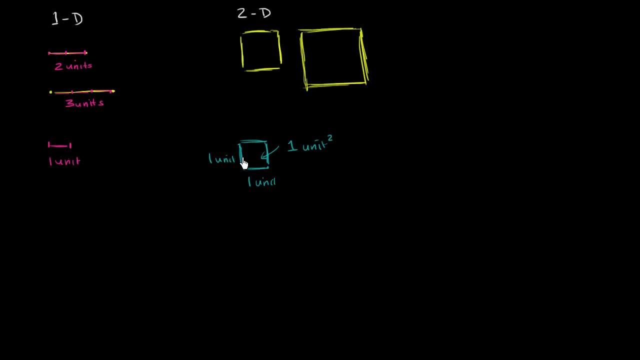 But now we can use this to measure these areas And we say: well, just as we said, how many of this unit length could fit on these lines, We could say how many of these unit squares can fit in here, And so here we might take one of our unit squares. 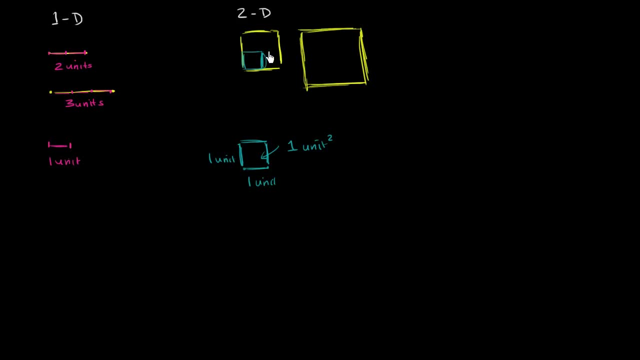 and say, OK, it fills up that much space, Well, we need more to cover all of it. Well, there, we'll put another unit square there. We'll put another unit square right over there. We'll put another unit square right over there. 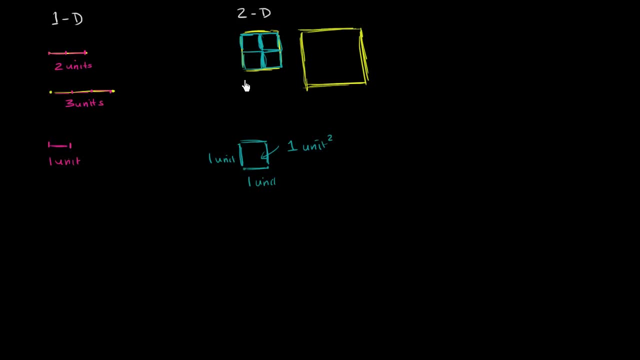 Wow, four unit squares exactly cover this. So we would say that this has an area of four square units, or four units squared. Now what about this one right over here? Well, here, let's see, I could fit 1,, 2,, 3,, 4,, 5,. 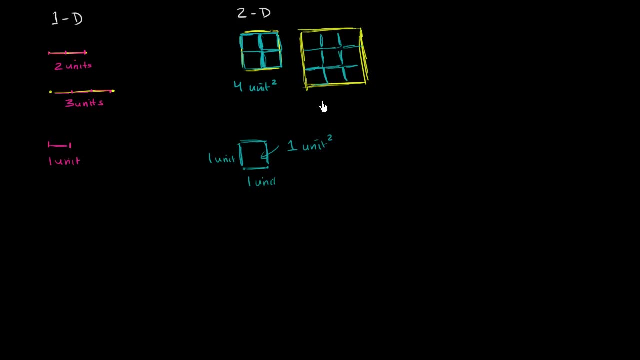 6,, 7,, 8, and 9.. So here I could fit 9 units squared. Let's keep going. We live in a three-dimensional world. Why restrict ourselves to only one or two? So let's go to the 3D case. 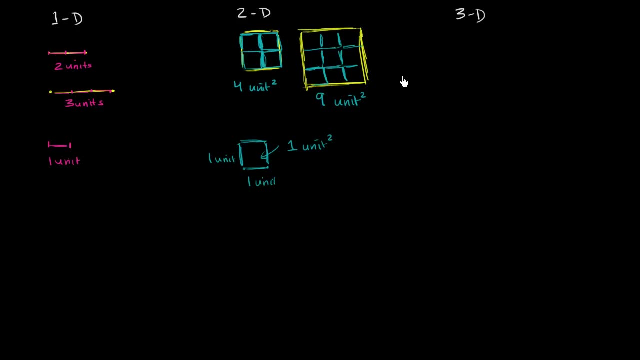 And once again, when people say 3D, they're talking about three dimensions, They're talking about the different directions that you can measure things in. Here there's only length, Here there's length and width, or width and height. 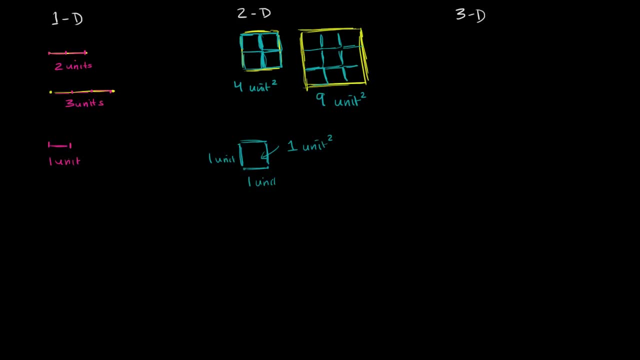 And here there'll be width and height and depth. So, once again, if you have, let's say, an object- and now we're in three dimensions, We're in the world we live in- that looks like this, And then you have another object that looks like this: 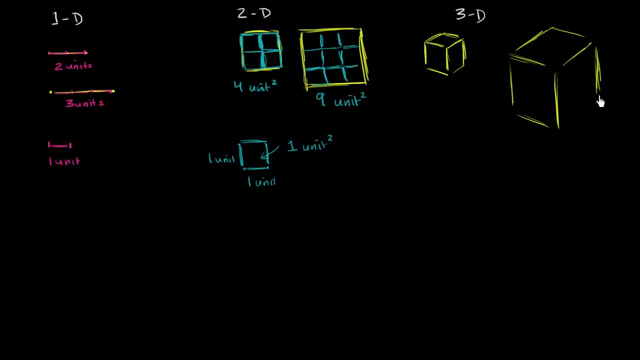 It looks like this second object takes up a third More space, more physical space, than this first object does. It looks like it has a larger volume, But how do we actually measure that? And remember: volume is just how much space something takes up in three dimensions. 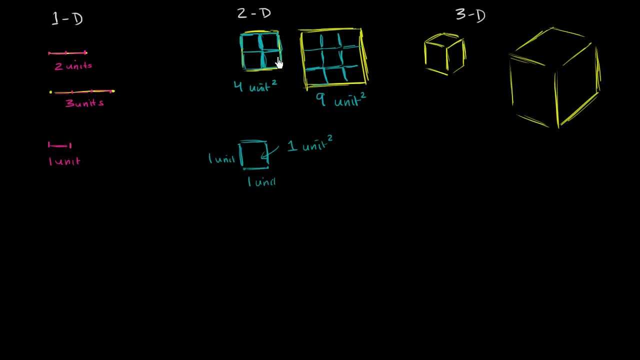 Area is how much space something takes up in two dimensions. Length is how much space something takes up in one dimensions, But when we think about space, we're normally thinking about three dimensions. So how much space would you take up in the world that we live in? 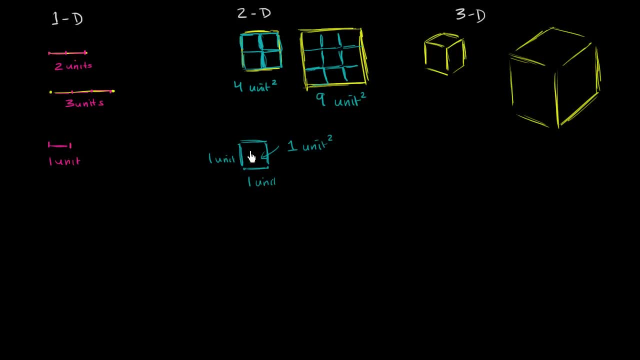 So, just like we did before, we can define, instead of a unit length or a unit area, we can define a unit volume or a unit cube. So let's do that, Let's define our unit cube. And here it's a cube, so all of its length, width and height. 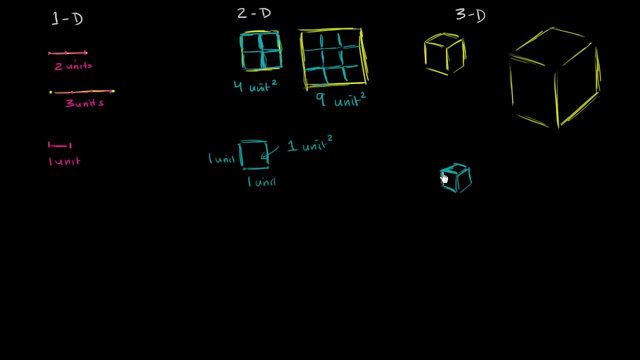 are going to be the same value. So my best attempt at drawing a cube, And they're all going to be one unit. So it's going to be one unit high, one unit deep and one unit wide, And so to measure volume, we could say well. 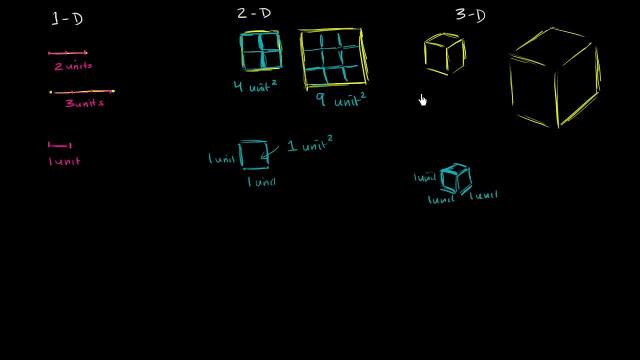 how many of these unit cubes can fit into these different shapes? Well, this one right over here, and you won't be able to actually see all of them. I could essentially break it down into, so let me see how well I can do this. 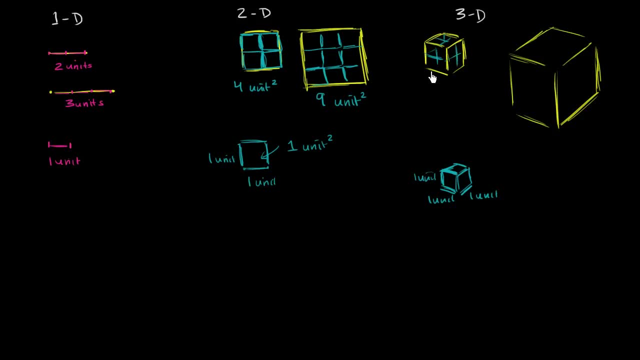 so that we can count them all. It's a little bit harder to see them all because there's some cubes that are behind us. But if you think of it as two layers, so one layer would look like this. One layer is going to look like this: 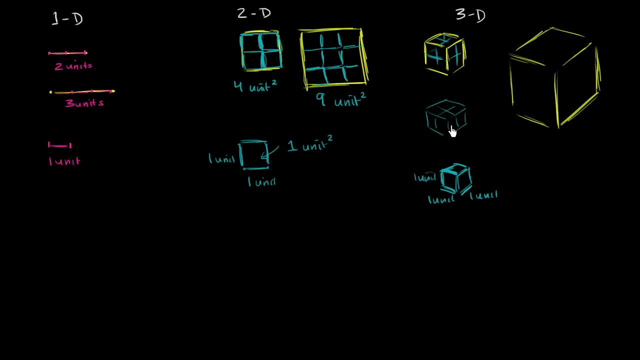 So imagine this. Imagine two things like this stacked on top of each other. So this one's going to have one, two, three, four cubes. Now this is going to have two of these stacked on top of each other. So here you have eight unit cubes. 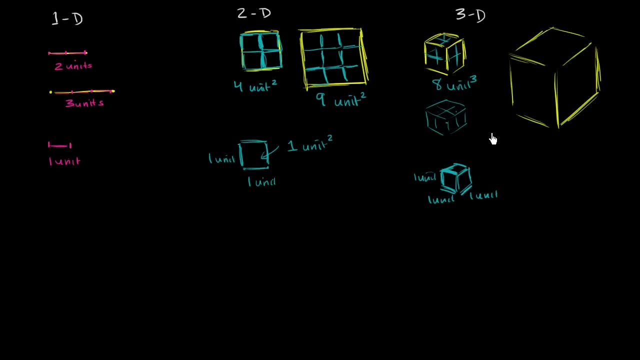 Or you could have eight units cubed volume. What about here? Well, if we try to fit it all in, let me see how well I can draw this. It's going to look something like this. Obviously, this is kind of a rough drawing.